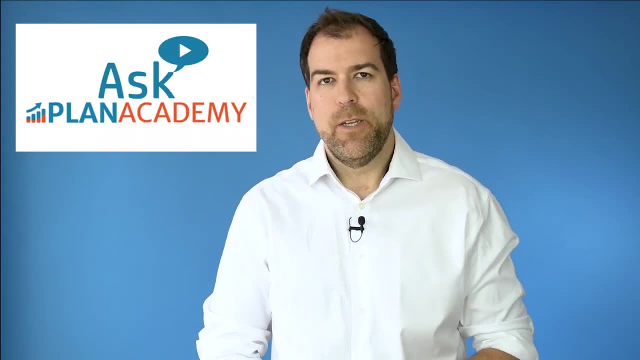 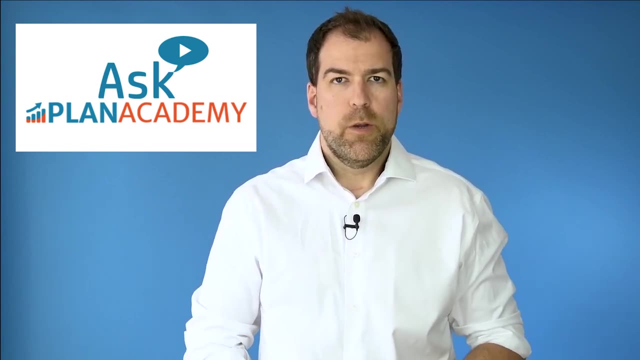 Hey everyone, it's Michael from Plant Academy. I want to welcome you back to another Ask Plant Academy video. I've been getting lots of questions recently about how to build good work breakdown structures for construction projects, So I thought in this video I'll take 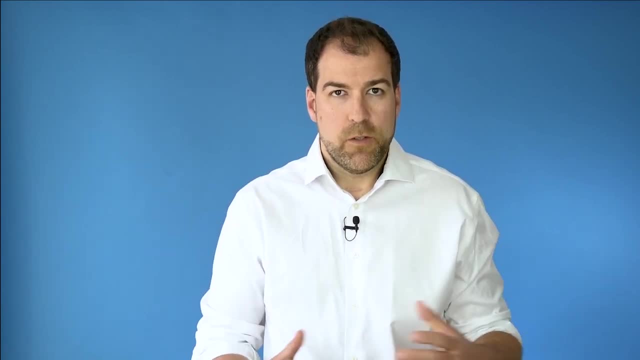 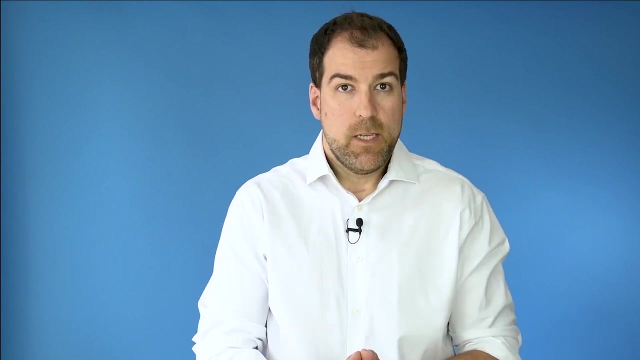 you through a few sample work breakdown structures for construction projects, and I'll also walk you through what I think is a really good generic work breakdown structure that should be used on most traditional construction projects. But keep watching, because I'll also show you where you can download some P6 templates, some of these work breakdown structures that we're covering today. 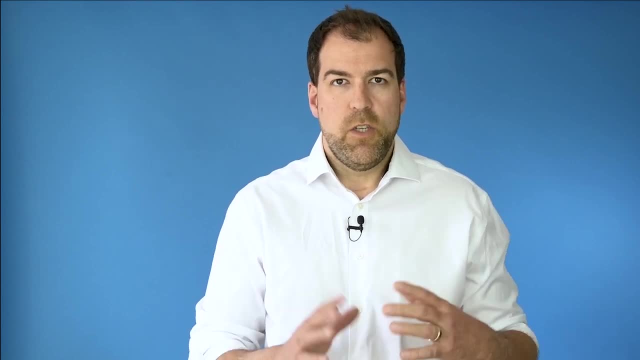 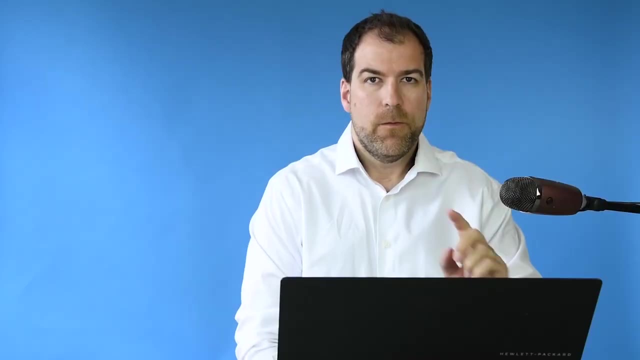 I'll show you how you can download those as templates to use as a starting point to build your own construction projects. Hey, if you're ready- I am too- Let's go. Okay, the first thing I want to show you here is a document, and this comes from the AACE, and this is their recommended. 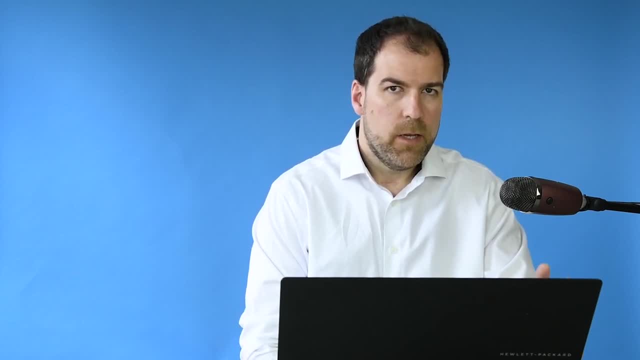 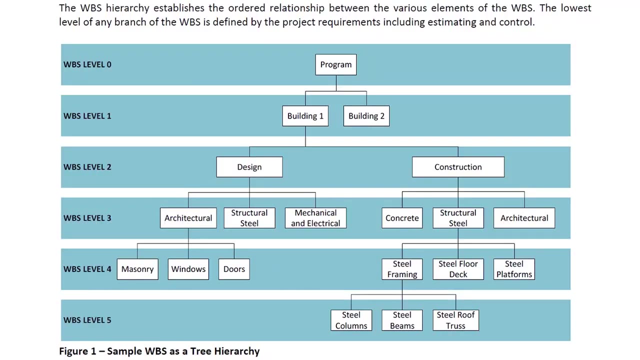 practice I'm developing the WBS and again there you can see that there's definitely a flavor that we're talking about construction projects here. So a couple things we want to highlight about this image here. Notice, on the left we have the different levels of the WBS. Okay, so at the 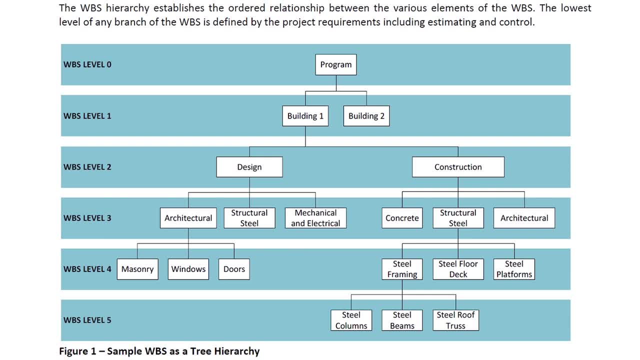 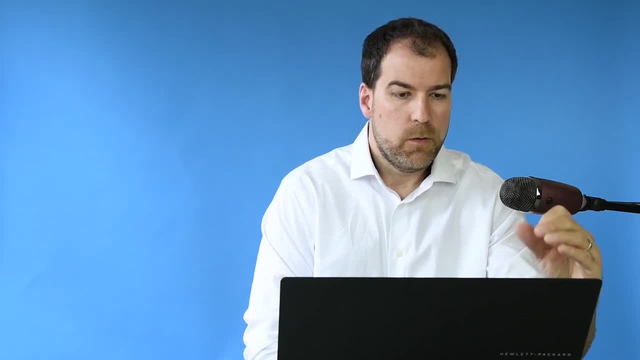 very top we have level zero. and that is here they're saying: that's the program, That can also be the project. Okay, so the project is always at level zero. Then we come down to record levels one through five. A really good question. as we develop our work breakdown. 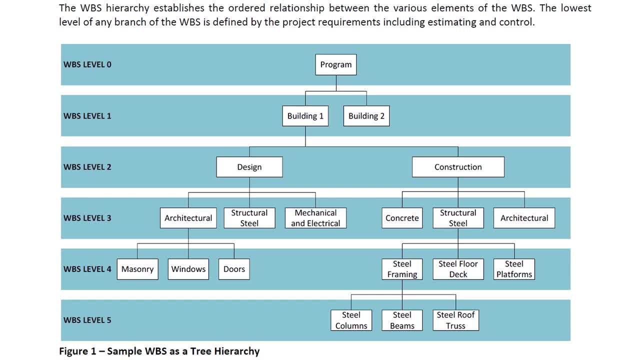 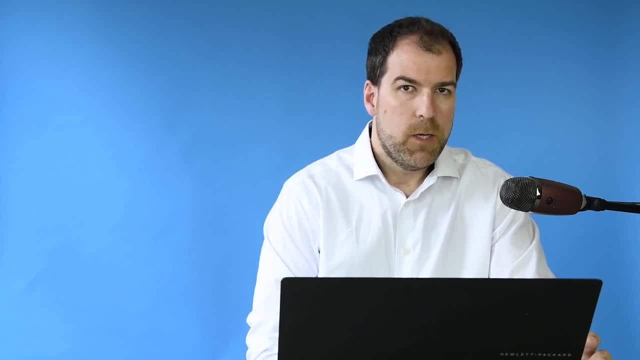 structure for construction projects is: how deep do we want to go? There is a possibility of going to deep. too deep will be too detailed, But of course it does depend on the breadth and the scope of your project. I like to go five to six levels deep If you're doing a major, mega build. 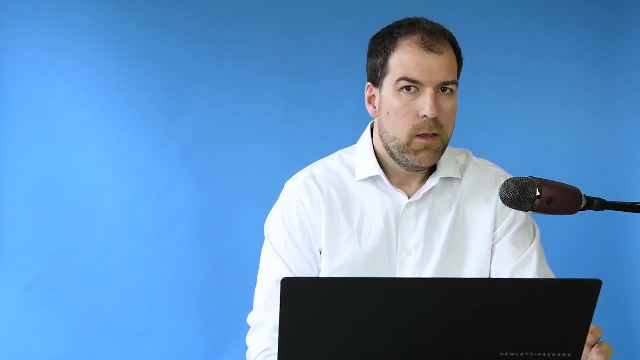 seven is more likely, But in my experience I haven't ever seen any project that's more than that. eight Doesn't mean it doesn't exist, but I haven't seen it. I like to be at level five for a typical one to two year project. That gives me lots of detail, but not too much, Okay. 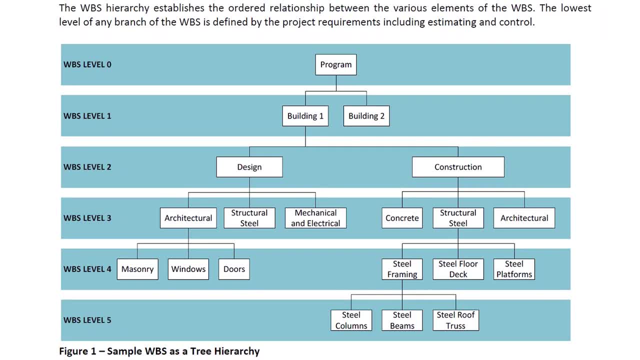 Now let's look at the structure here. Of course, you understand the concepts behind work breakdown structure- that we're taking the work, the scope of the project, and we're breaking it down into smaller and smaller chunks- right. And the question is, how do we do that? There is some. 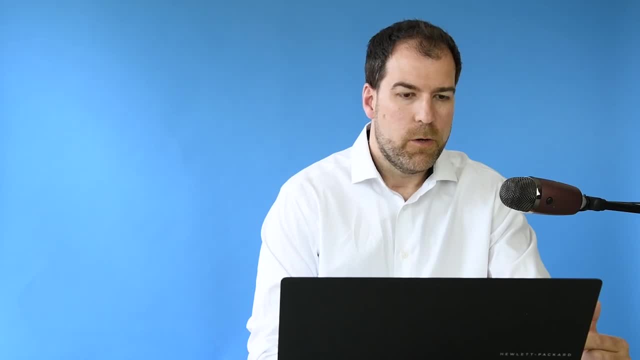 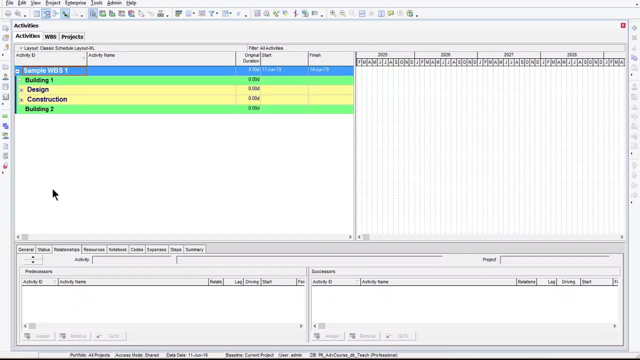 intelligence that goes into the right way to do it for construction projects. Okay, So we're going to get to that. right now I'm going to flip over to Primavera P6 and let's have a look at a couple samples in Primavera P6.. Okay, Here's the first work breakdown structure we're going to look at. 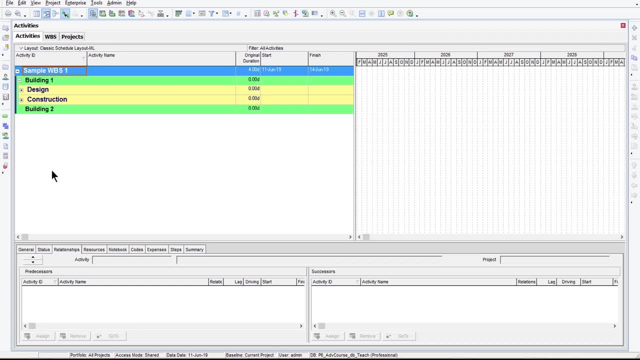 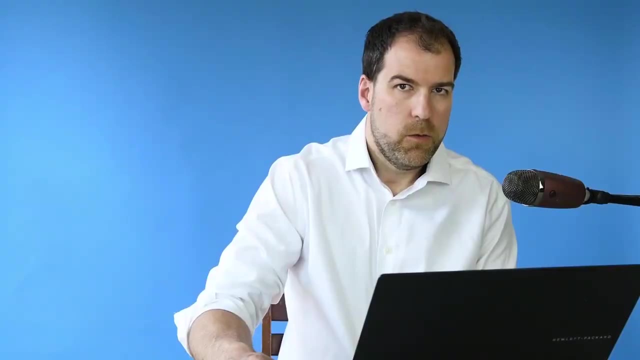 As you can see, let's talk about how we take the work and we break it down. This is the same work breakdown structure we just saw in the image before. So up at the top, here's our level zero Sample. WBS is our level zero. Next we're breaking it into building one and building two. 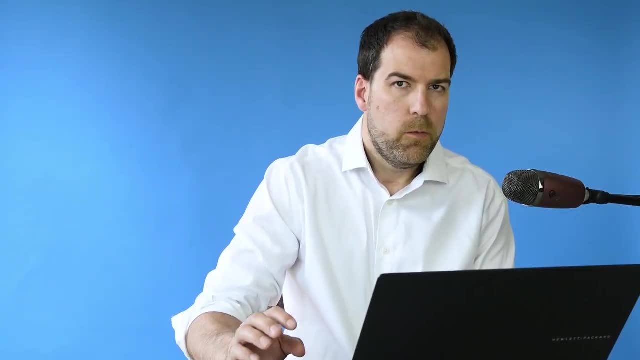 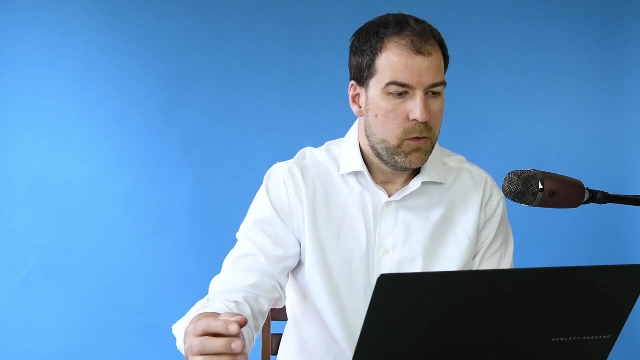 Okay. So this is the large pieces of work. We have building one and building two, which could also be area one, area two, or phase one, phase two- Okay, Those also work. And then underneath we're adding design and then construction. 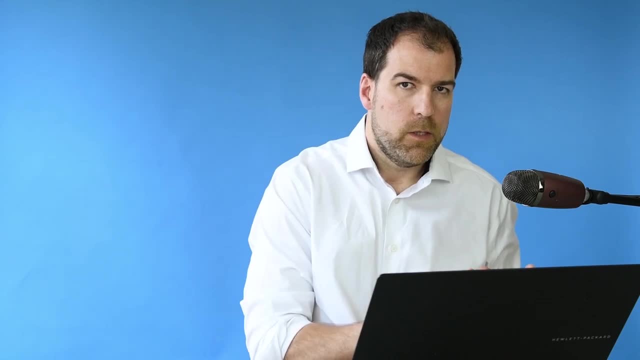 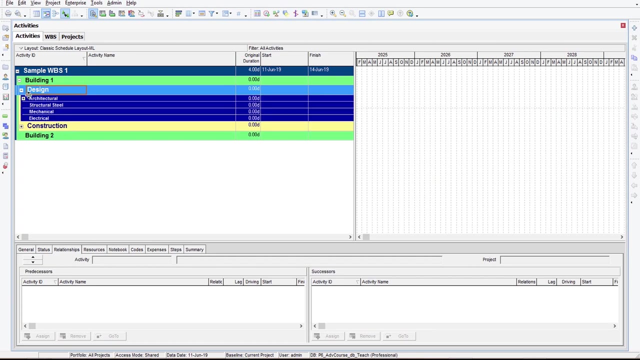 So we're breaking those two apart. We're putting all the design activities in one area. We're putting all the construction activities in another area. Now, if you have to break your design work down further because there's a lot of it in your project, then, as you can see, we've broken our design. 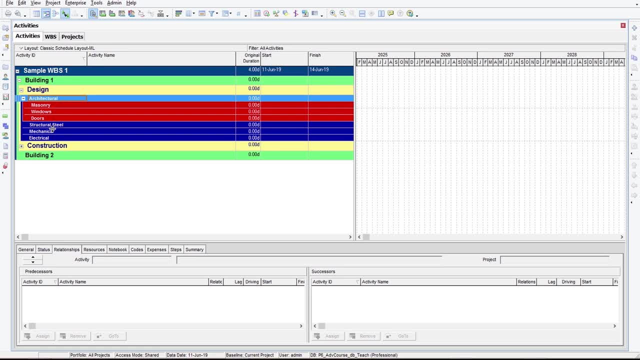 work into the different components, Again, architectural, structural steel. So those are getting into sort of my big disciplines and then even smaller work packages underneath. Let's look at construction. I'll just roll design back up. Let's look at construction. 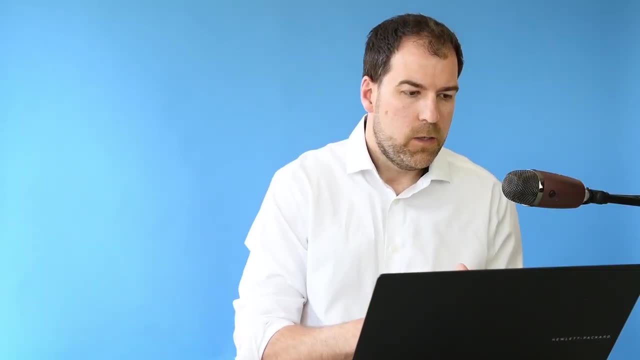 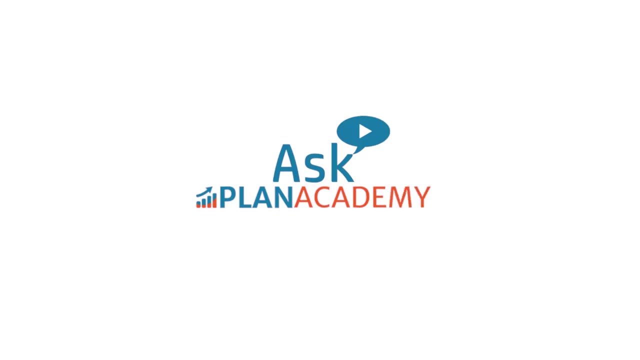 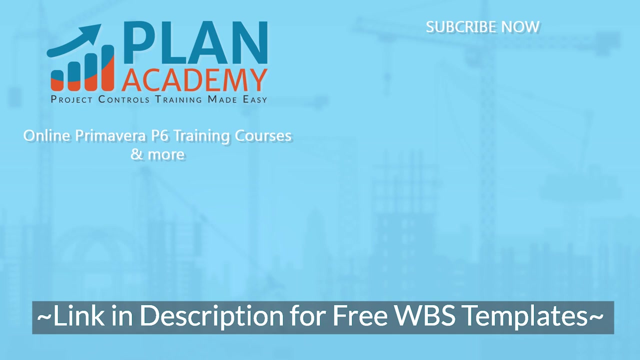 Construction same thing. We've taken construction and we've broken it into our disciplines and then into our sub-disciplines or our work packages. Want to see more examples and grab those free templates? Just click the link below the video. Thank you so much for watching. I'll see you in the next video.